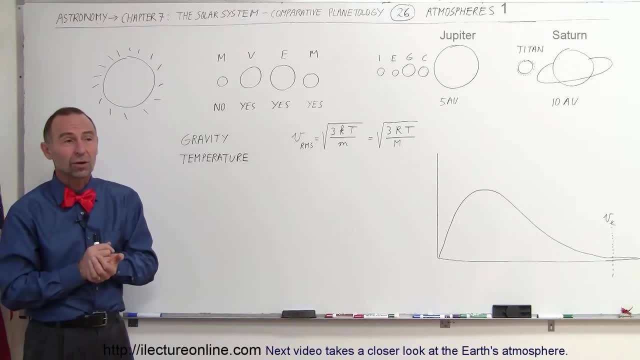 velocity of the Earth is somewhere around 7 miles per second. So 500 meters, that's about a third of a mile or so. that's not nearly fast enough. However, it turns out that the distribution curve of the velocity of molecules is not a narrow band. it's kind. 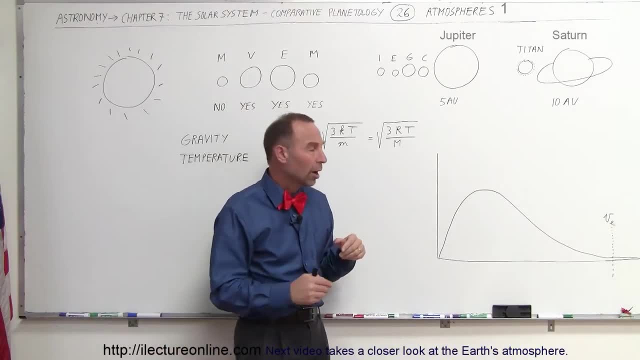 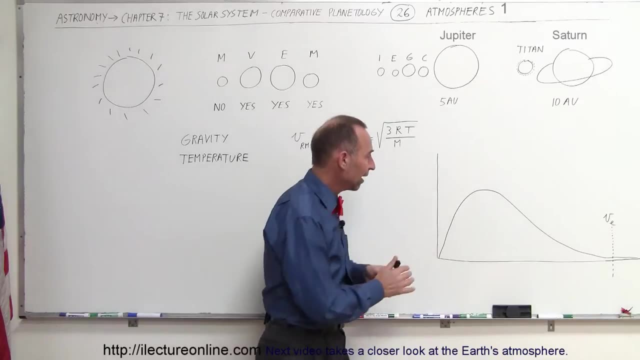 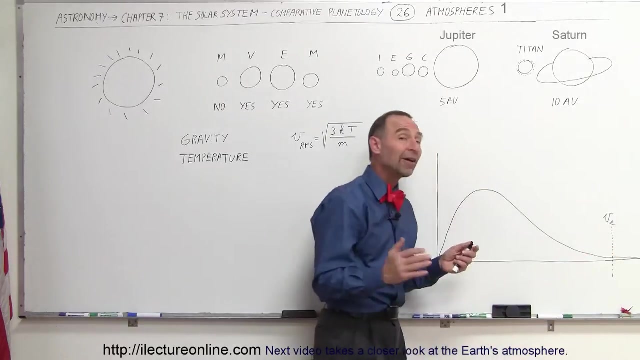 of a wide distribution. This is called a Stefan-Boltzmann distribution of molecular velocities, velocities of molecules in the atmosphere And if, and you can see that the vast majority of molecules are about the same amount of velocity, but there's some- not very many- that move quite a bit faster because of all. 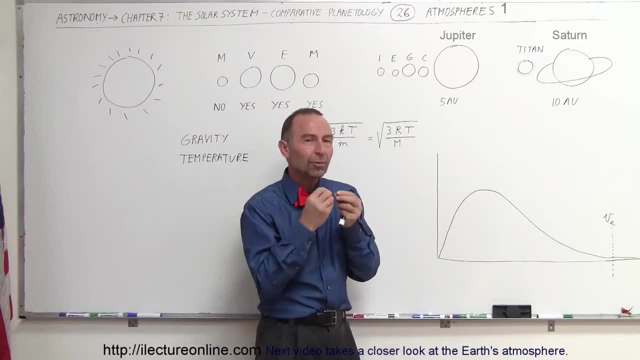 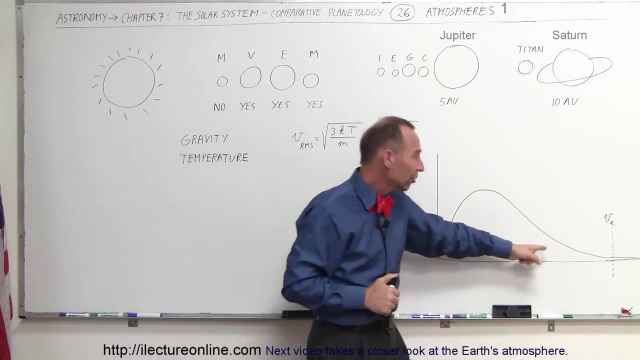 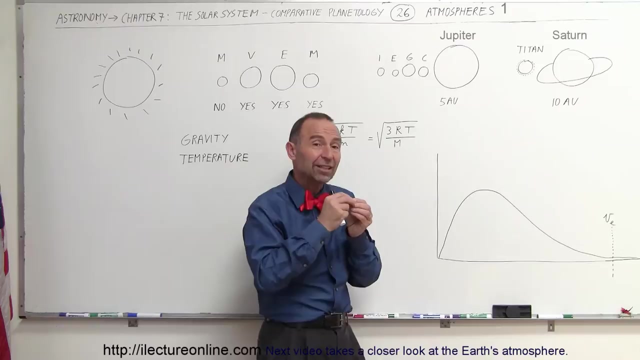 the bouncing around, the molecules hitting each other, colliding, Some of the molecules can reach some very high speeds, and when those molecules are very high up in the atmosphere and they reach really high speeds, sometimes they can actually exceed the escape velocity of the planet, in this case the Earth, and so those molecules would actually then get. away from the Earth and you couldn't pull them back. Luckily, the Earth is a big enough planet with a strong enough gravitational field that very, very few molecules will ever leave the Earth, and so the atmosphere is still very rich, very thick here on the Earth, and so we need that atmosphere to live and to be protected. Venus has an atmosphere. Mars has an atmosphere, but not a very thick atmosphere. The density of the atmosphere on Mars is less than 1% the density of the atmosphere of the Earth. What happened to the atmosphere? Well, most of the atmosphere has leaked off The reason. 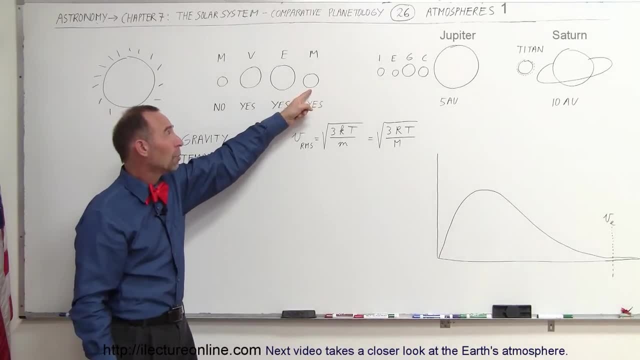 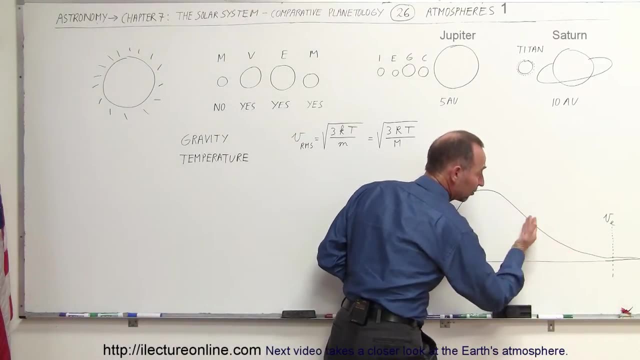 for that is, the gravitational force is much smaller on Mars compared to the Earth or Venus, and so, therefore, with an escape velocity that's much to the left – a much lower velocity – you can see that many more molecules wouldn't reach the speed to get away from the planet. and therefore most of the atmosphere on Mars has indeed leaked off. Mercury being so small – it's very small, it's only about 1, 20th the mass of the Earth – the gravitational field is a lot weaker and therefore Mercury simply does not have any atmosphere left. It's all leaked off into space. the escape velocity was much too low, So very many molecules have leaked off and for a long time already mercury has not had an atmosphere. But there's a second factor: the temperature. 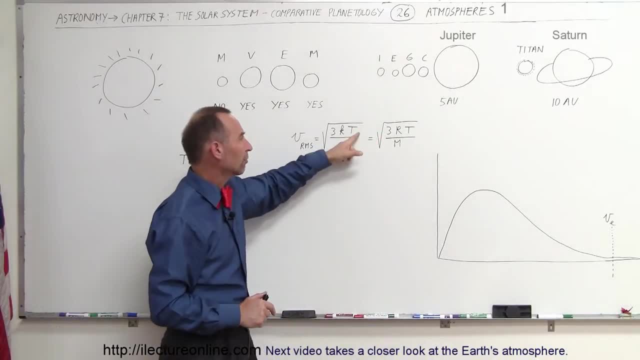 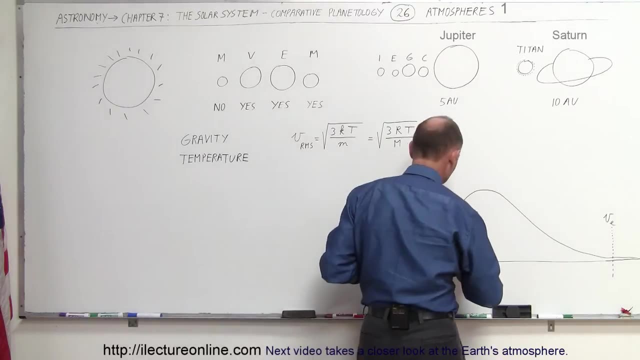 Notice that the speed of the molecules do depend on the temperature. The temperature goes up, the speed increases. So what happens is, for a location like mercury, where the temperature is hotter, what would happen is that the molecules would be distributed far, much farther to the right, and you can 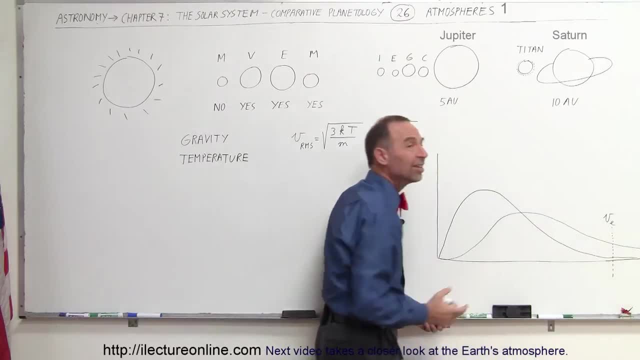 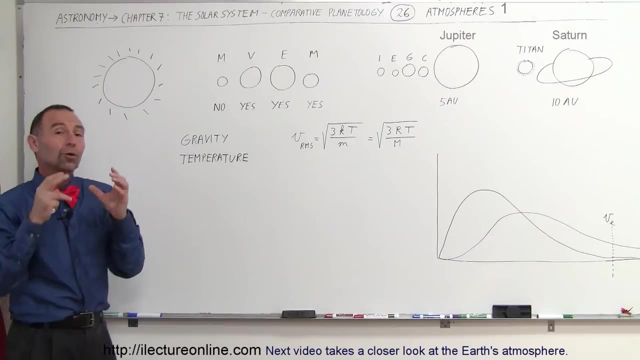 then see that a much greater percentage of the molecules would exceed the escape velocity, In this case for mercury, and so that's one of the reasons why mercury no longer has an atmosphere. Not only does mercury have a small mass and not a very strong gravitational field, it 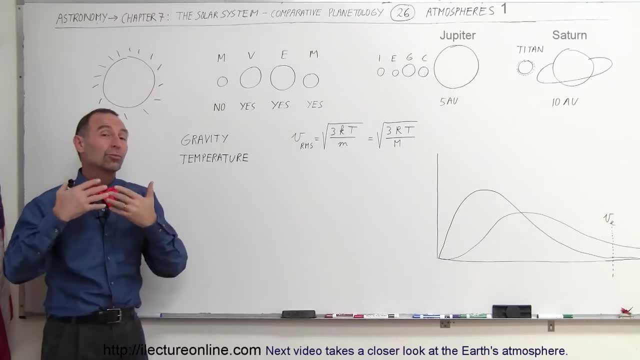 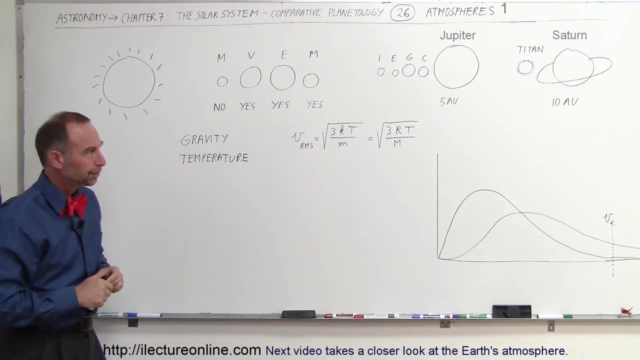 has very high temperatures, being very close to the sun, therefore molecules moving much faster. So mercury got hit by double whammo. It's not big enough and it's way too hot. no atmosphere Now when you go out further out in the solar system. here we have Jupiter with the four large moons: Io, Europa, Ganymede and Callisto, And none of those four moons, None of those four moons have an atmosphere, Not even Ganymede, which is the largest moon in the solar system, larger than mercury. 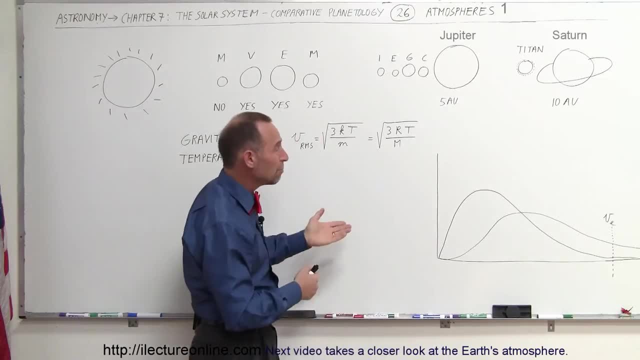 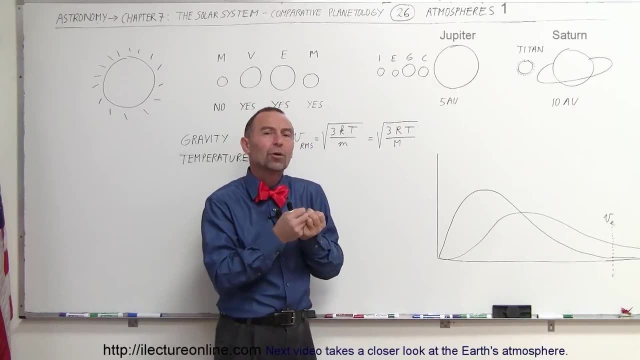 and it is much farther away from the sun, so much cooler. So the molecules on Ganymede, if Ganymede had an atmosphere, would not be moving nearly as fast, And so we would expect some of those to stay behind. but it looks like Ganymede has no. 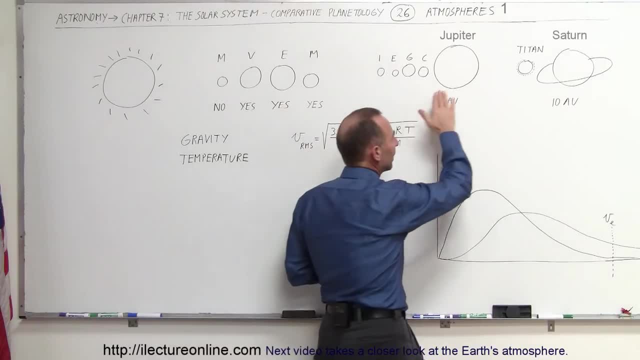 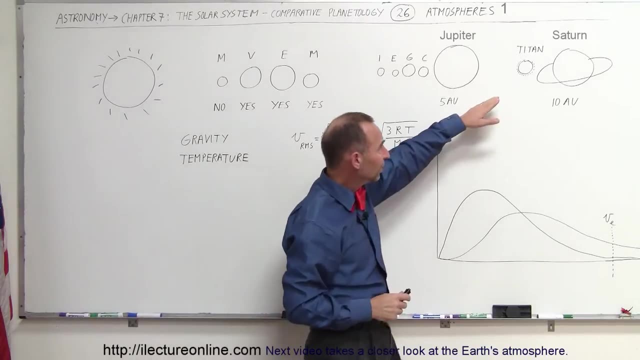 atmosphere at all. But what is interesting is if we go further out in the solar system, at ten astronomical units, where we find the planet Saturn, Saturn, We can see that the largest moon of Saturn, Titan, which is almost as big as Ganymede. about the same size as Mercury, Titan does have an atmosphere. Now, why does Titan have an atmosphere and Ganymede does not? Well, Titan is twice as far away from the sun as Ganymede. It's much colder where Titan is. Molecules would be moving much slower And because of that that made all the difference in the world. So about the same size, About the same gravitational force, Holding atmosphere. But Ganymede does not have an atmosphere because it's too close to the sun. Molecules move too fast and they've leaked off Titan. the molecules are much are moving much slower because it's much farther away and Titan was able to hold on to his atmosphere. There's, of course, other factors. What was the consistency of the atmosphere when the, when the moons were first formed? 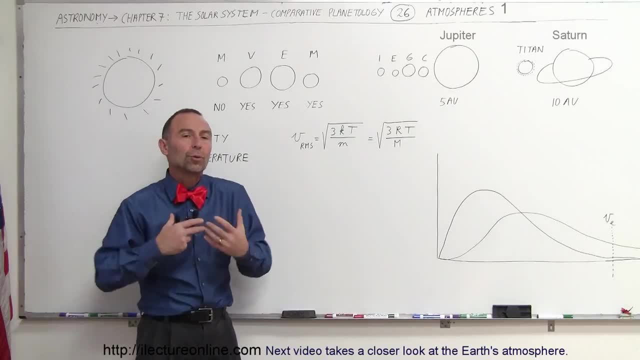 the planets were first formed, And it could be that Titan was much more rich in in the kind of compounds that make up the atmosphere. Remember, as we saw in a few videos ago, That the predominant constituent in the atmosphere of Titan is actually methane. And maybe there might not have been a lot of methane where Ganymede was when Ganymede was formed and therefore it doesn't have an atmosphere. So there could be other factors, But at least the the two main reasons why an atmosphere exists is gravity and temperature. 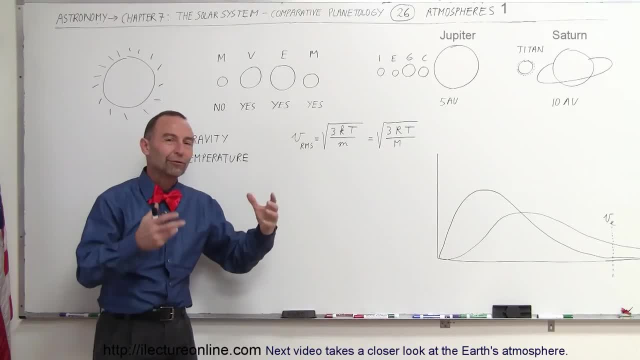 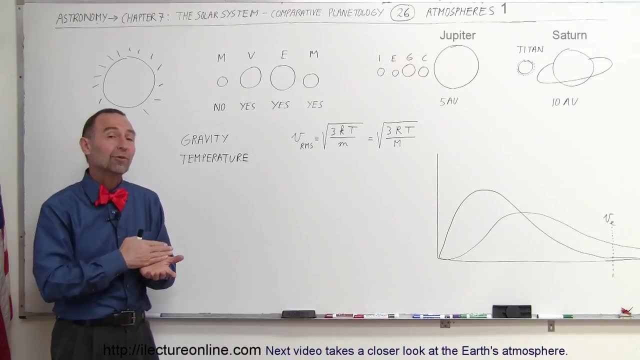 And for Titan, it had enough gravity and it was cold enough for it to be able to hang on to its atmosphere. And so that's how we study the, the reasons why planets and moons have atmospheres or do not have atmospheres, And it's based upon those two main principles. 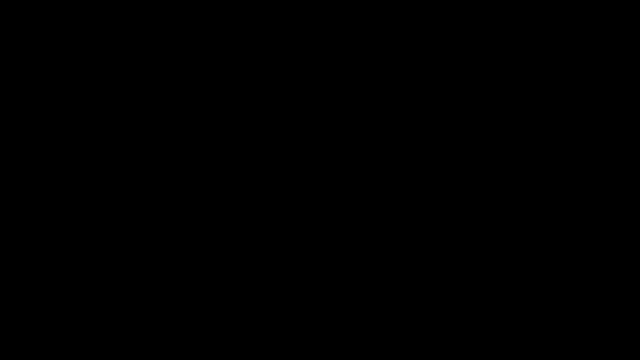 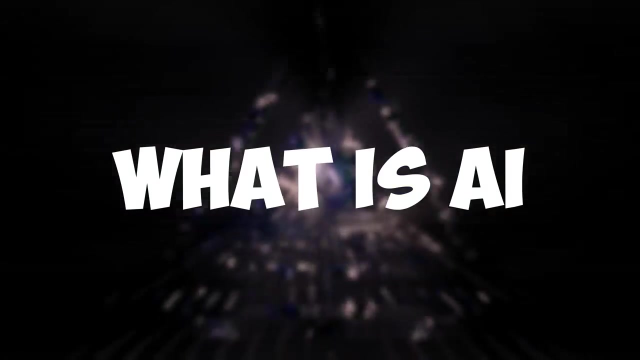 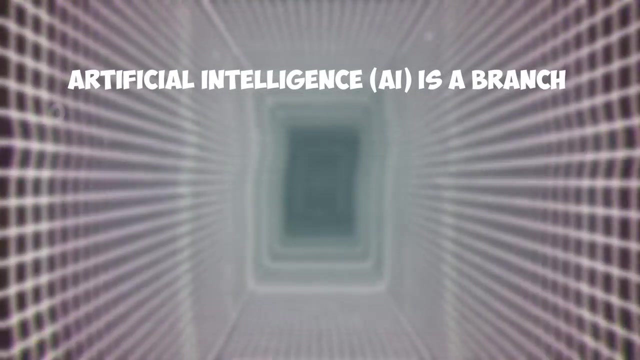 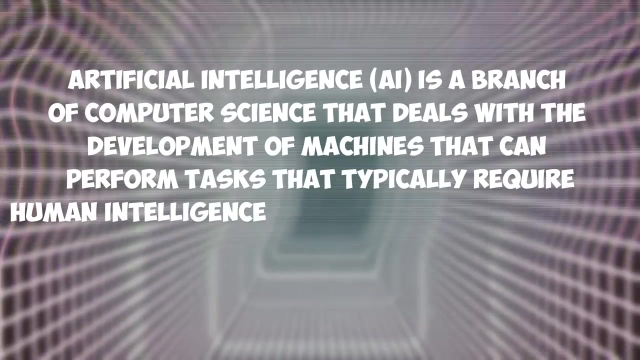 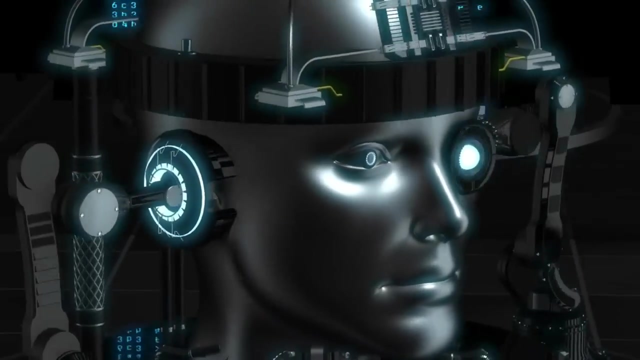 Artificial Intelligence is a branch of computer science that deals with the development of machines that can perform tasks that typically require human intelligence, such as visual perception, speech recognition, decision-making and language translation. The goal of AI is to create intelligent machines that can think, reason and learn like humans. 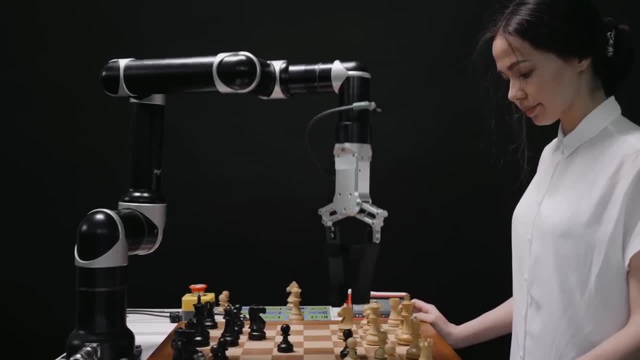 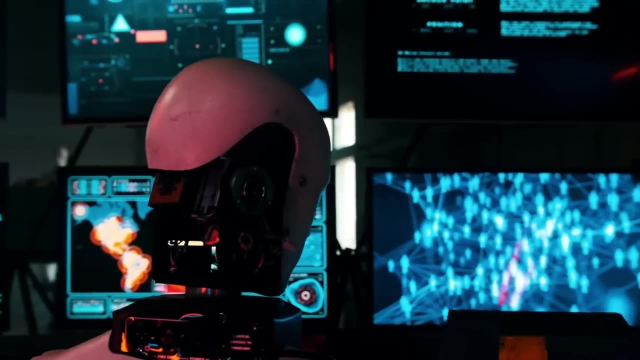 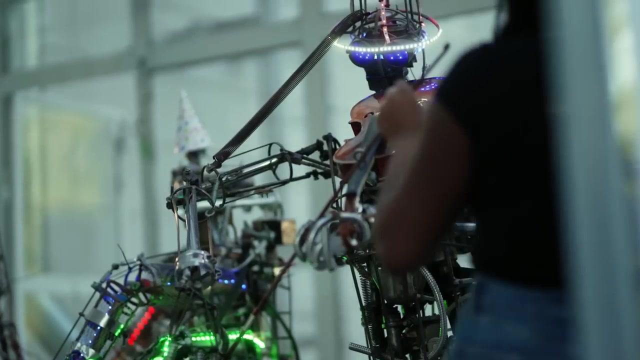 These machines are designed to mimic human cognitive abilities and make decisions based on data, algorithms and statistical models. AI has the potential to revolutionize many fields, including healthcare, finance, education and transportation. It has already led to significant advancements in areas such as speech recognition, natural language processing and computer vision.